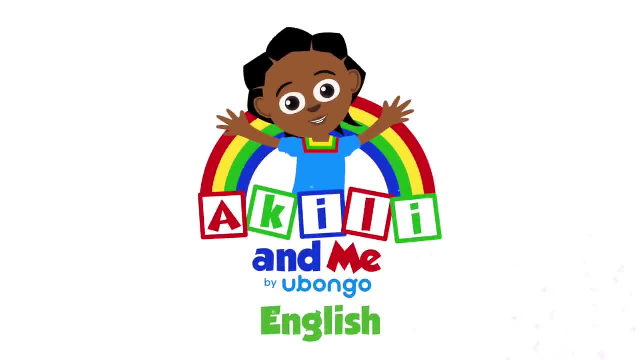 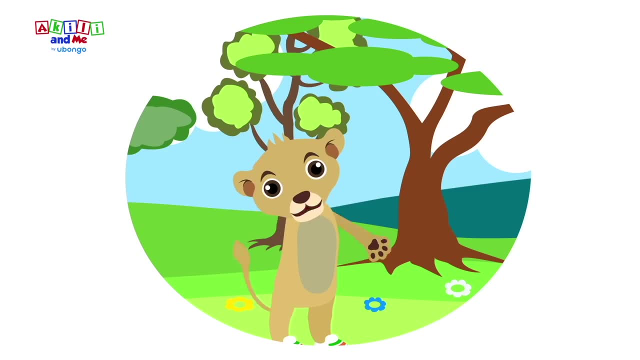 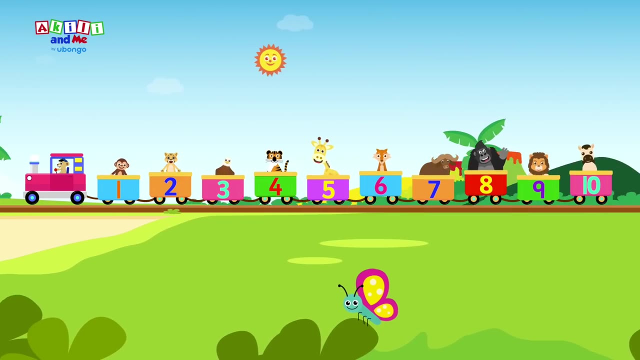 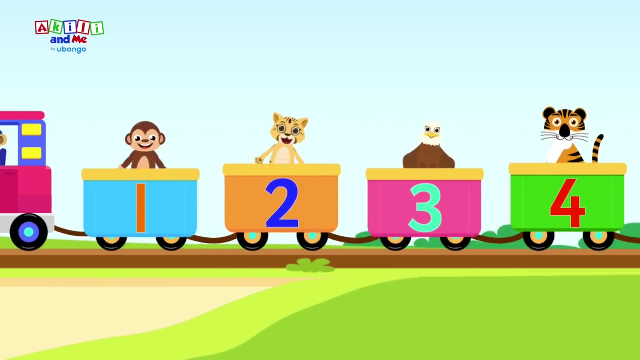 A-kiri, a-kiri, a-kiri, a-kiri, Boop-dee-doo, Flip one, flip two. I just love to count with you. Let's go. Numbers, numbers, numbers, Numbers are fun. 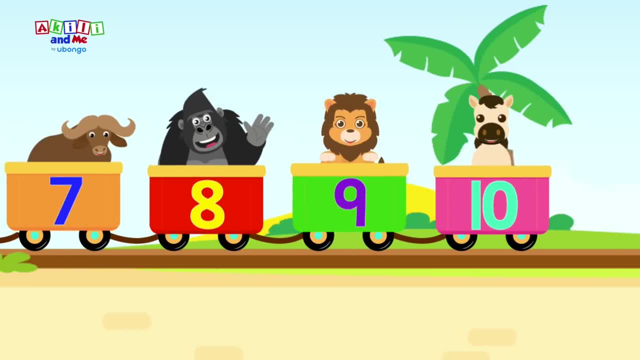 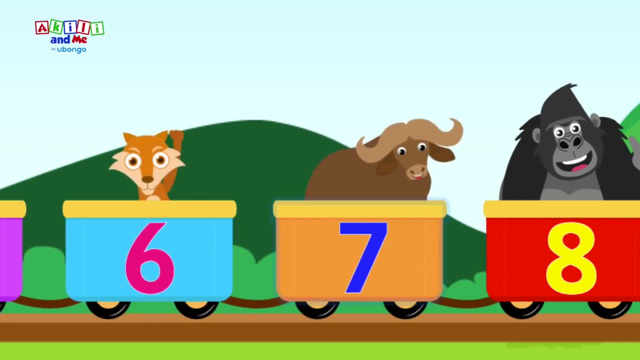 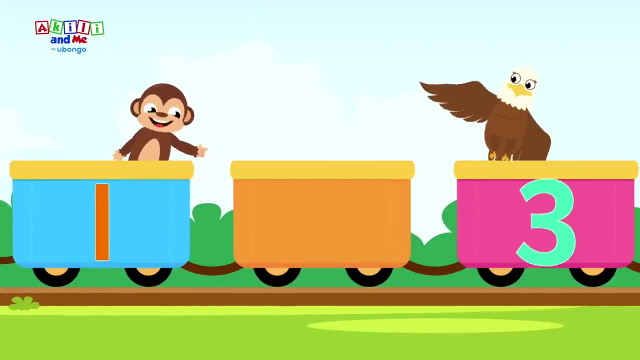 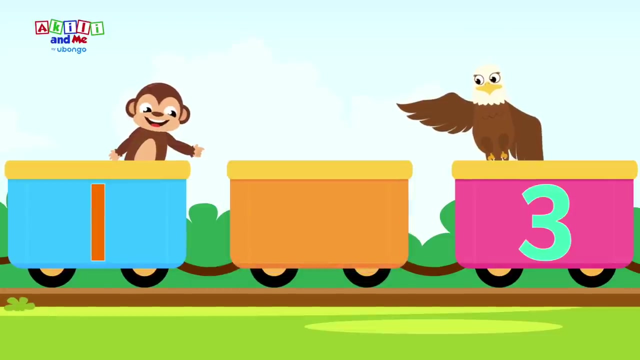 Numbers, numbers, numbers, Numbers are fun. One, two, three, four, five, six, seven, eight, nine, ten, One, three, Hmm, there's a number missing here. What number is missing? Let's count from the beginning to find out. 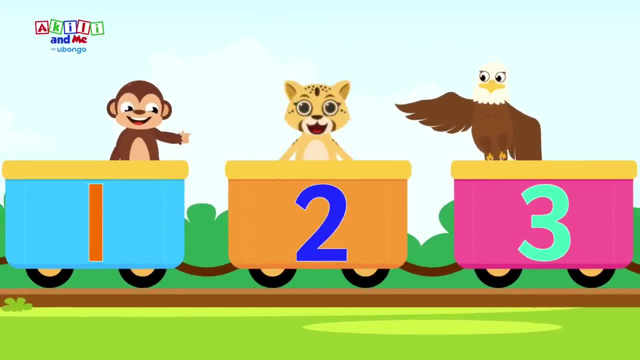 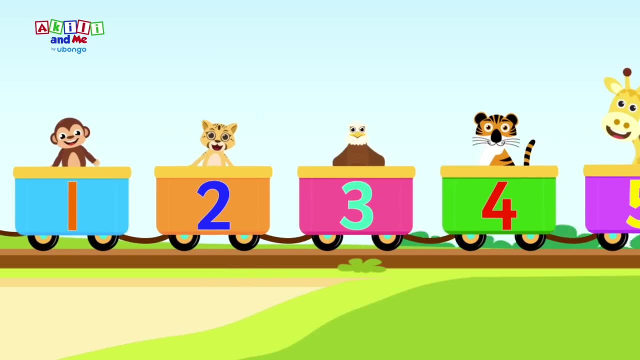 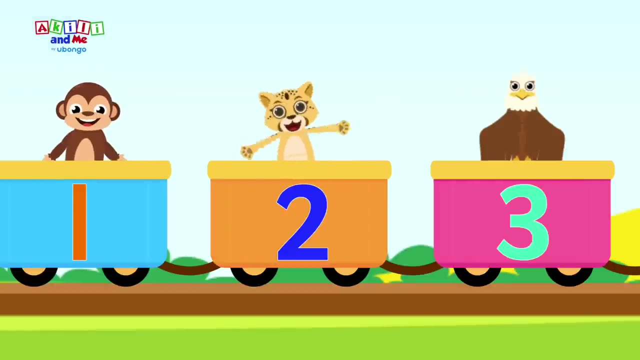 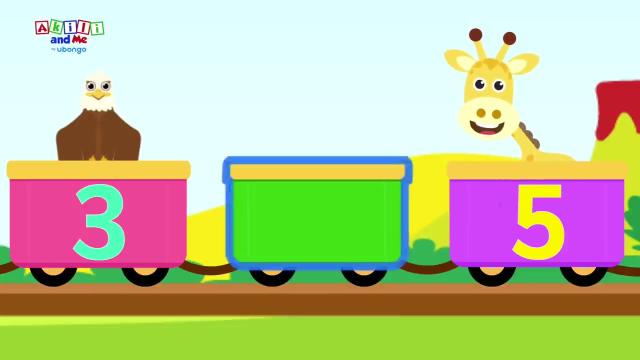 One, two, three. Yes, number two was missing. One, two, three, four. Numbers, numbers, numbers. Numbers are fun, Numbers, numbers, numbers, Numbers are fun. One, two, three, five. Hmm, there's a number missing here. What number is missing? 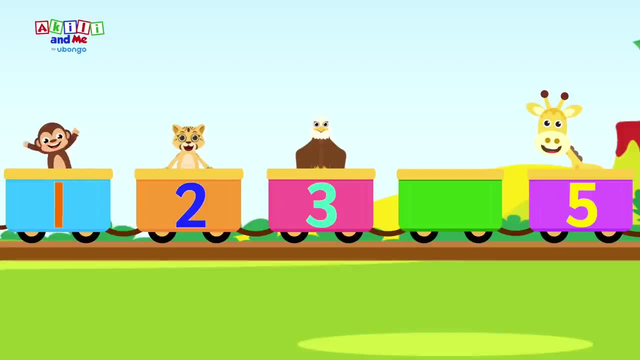 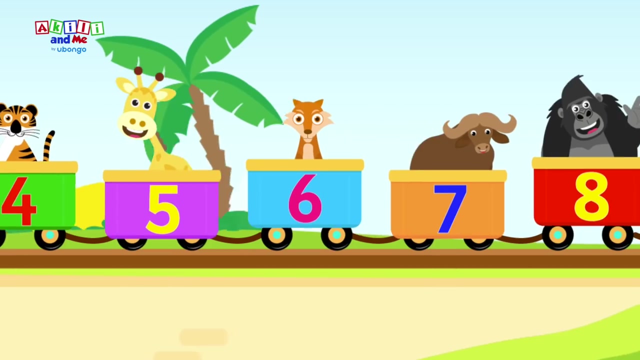 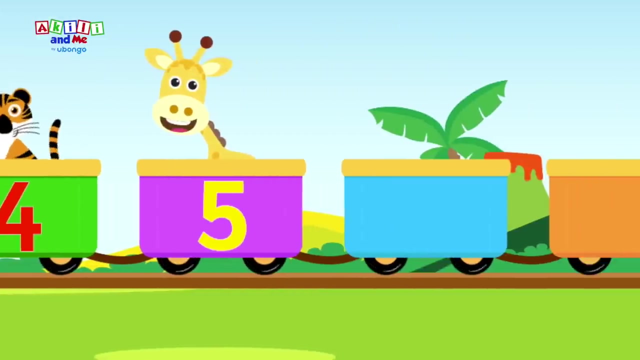 Let's count from the beginning to find out: One, two, three, four, Five. yes, number four was missing. Numbers, numbers, numbers. Numbers are fun. Numbers, numbers, numbers, Numbers are fun. One, two, three, four, five, eight, nine, ten. 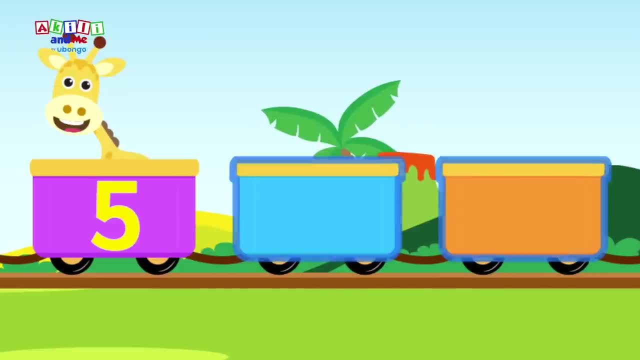 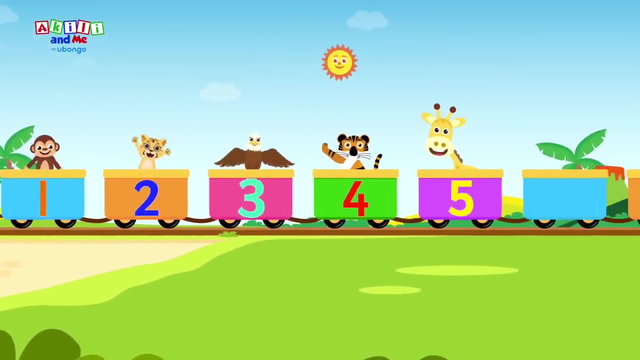 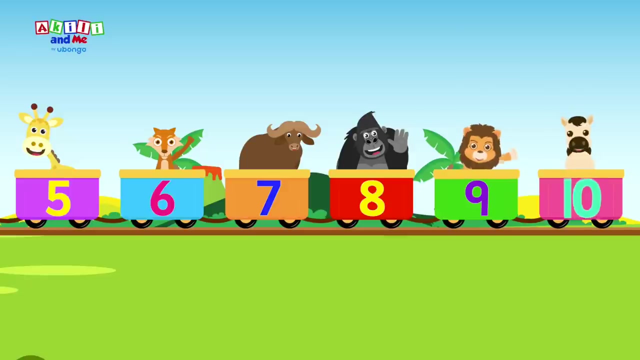 Hmm, there are two numbers missing here. Let's count from the beginning to find out What numbers are missing: One, two, three, four, five, six, seven, eight, nine, ten. Yes, number six and number seven were missing. 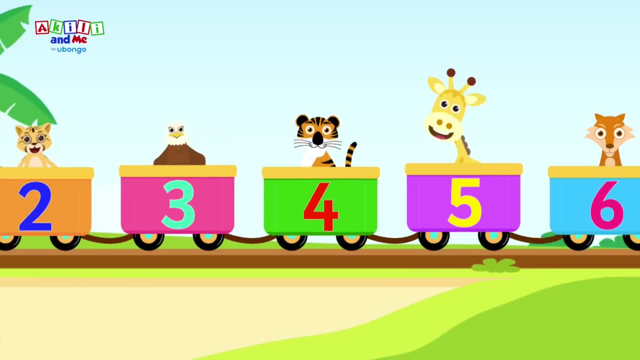 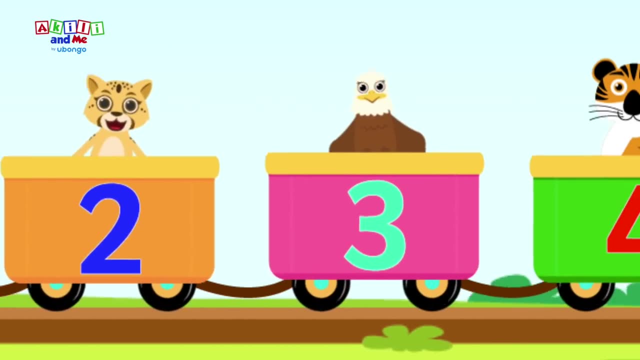 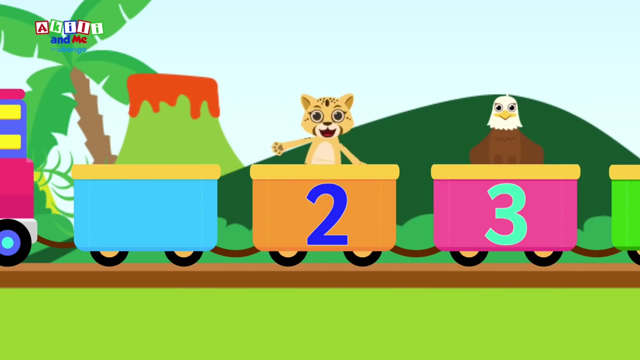 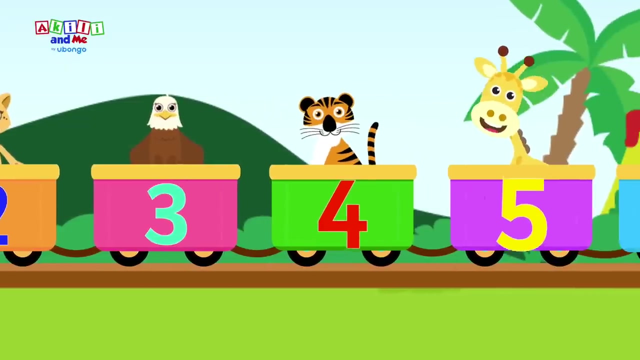